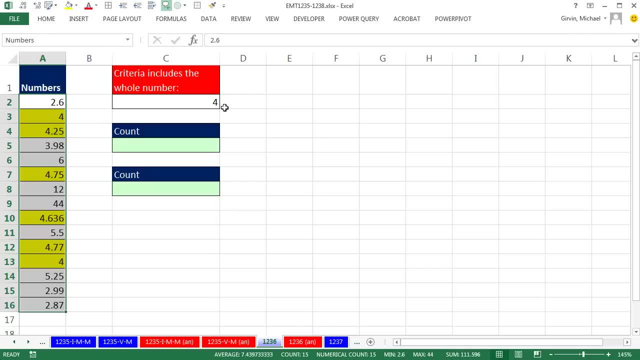 And we need to count all the numbers that have an integer 4.. Now we should include 4,, 4.25,, 4.75, and all of these numbers. If we happen to have a number like 14, we do not want to include that. 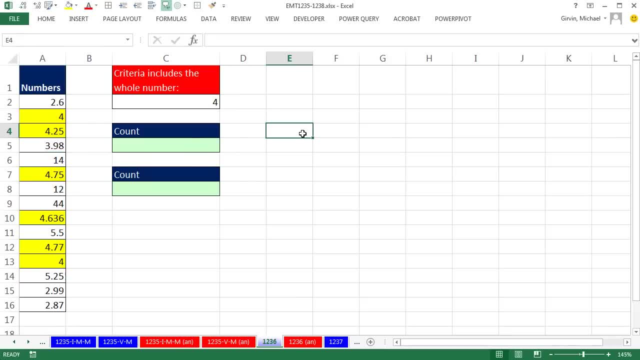 So, in essence, our criteria is going to be something like this: Greater than or equal to 4 and less than 5.. Now the way we're going to get less than 5 is we can say less than 4 plus 1.. 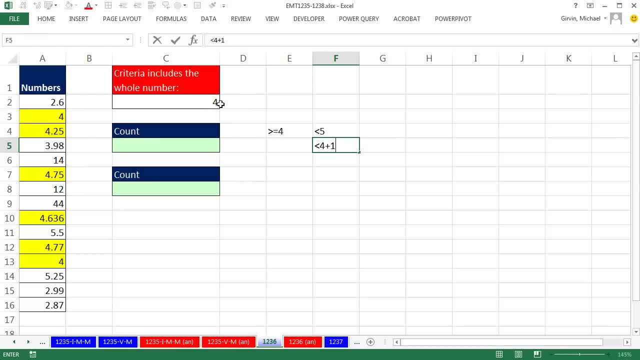 Now, that's because we want to have a single input here so we can change it and instantly we get a count. For example, if I put a 2 here, I should be getting a count for a 2,, a 2, and a 2,, so 3.. 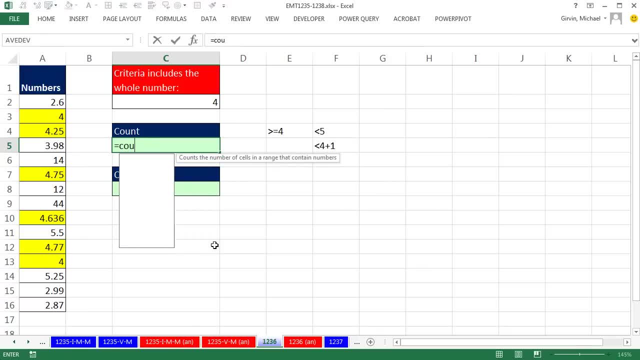 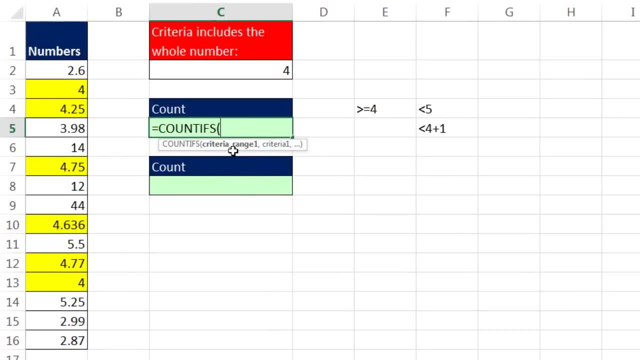 All right. so counting with two conditions sounds like the perfect job for the COUNTIFS function. It has a criteria range- that's the whole range, and then a criteria Notice. it says 1, 1.. So our first condition will highlight the entire range. 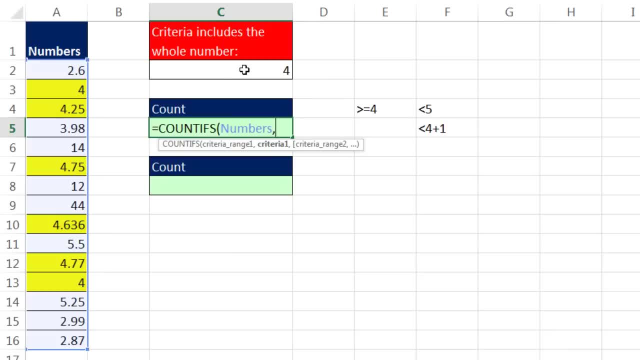 comma And the criteria. well, I want to link it to the cell, So I'm going to put: oh, I can't just click on it because it would put the 4 in there And I need the comparative operator before it. 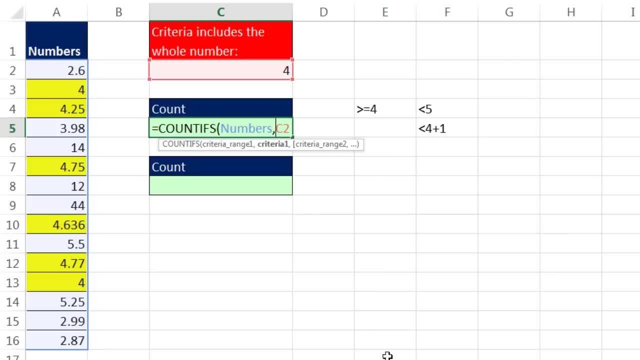 And guess what? The comparative operator has to be in double quotes, So double quotes greater than or equal to, And in Excel you have to put two operators like that: End: double quote. Now, this won't work. You can instantly see the form is not working. 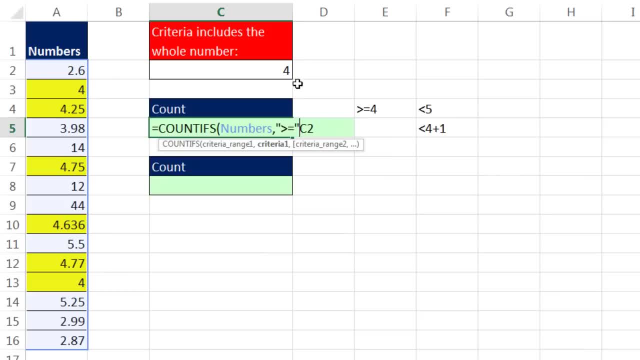 because that blue cell turned black. We need to join the comparative operator and the cell reference with our condition or criteria. You use the ampersand the and symbol Shift-7.. So that will work. You could actually highlight that whole constructed. 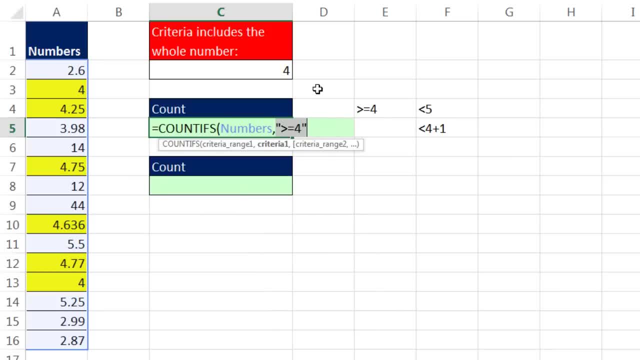 criteria and hit the F9 key to evaluate, And you'll see that, sure enough, it will evaluate to the correct comparative operator and number. Now I'm going to Control-Z because I want to leave it connected to that cell comma. And now the second criteria: notice it's a criteria range 2. 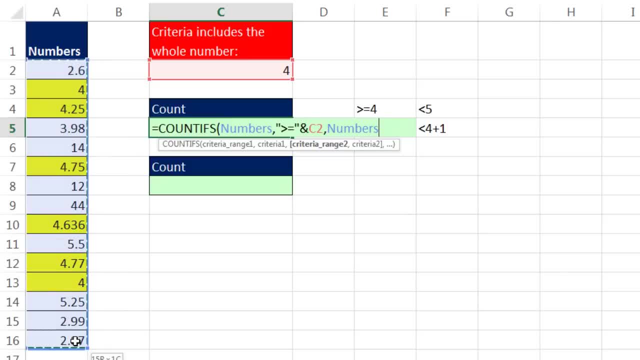 and criteria. All right, Criteria. 2. We highlight the same exact range comma in double quotes, less than in double quotes, and join it to Shift-7, whatever we type there plus 1.. Now the way that Excel calculates formula. 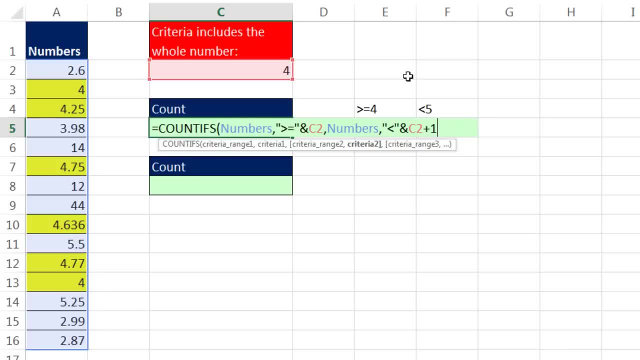 that math operator actually gets evaluated before the ampersand, So it will add and get 5.. If we highlight this criteria 2 here and hit the F9 key, you can see, sure enough, we get the correct answer, Control-Z, and that formula will work. 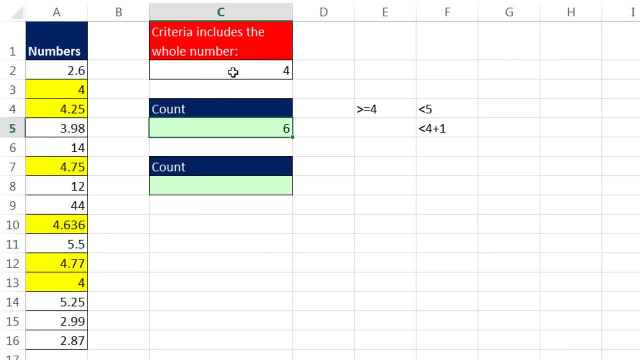 Close parentheses, Control-Enter, and we get a 6.. If I change this up here to a 2,, instantly I get a count of 3.. Now there is another way, and I'm sure there's actually many ways we can do this. 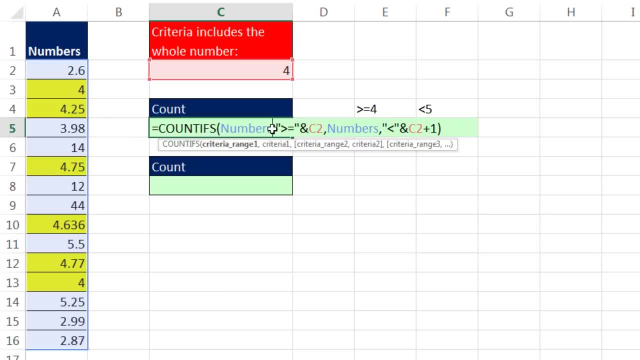 Count Ifs is almost always the fastest calculating method. The comparative operators sometimes get a little tricky, but usually that is the fastest way. Usually, that is Count Ifs is the best way to go Now, if you actually didn't have Excel 2007 or later. 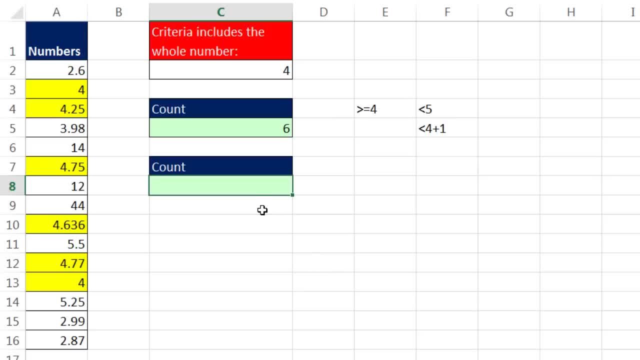 which is kind of unlikely in this day and age, although some people still have 2003 and earlier. you couldn't use Count Ifs, So we'd have to construct a different type of formula, And I'm going to start off with the integer function. 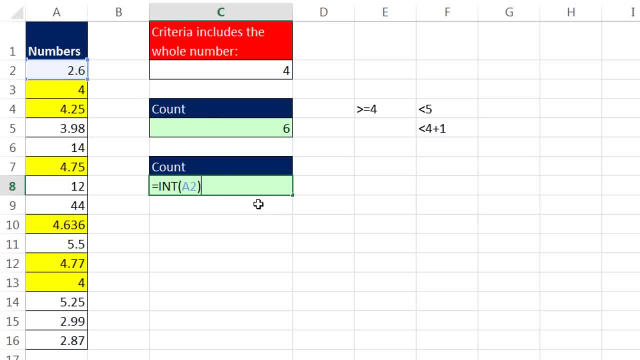 Now the integer takes a number and if I just close parentheses and highlight this in F9, you could see: oh, it just takes the integer. It actually always rounds down. So 2.6 becomes 2,, 4 would become 4,, 4.25 would become 4, Control-Z. 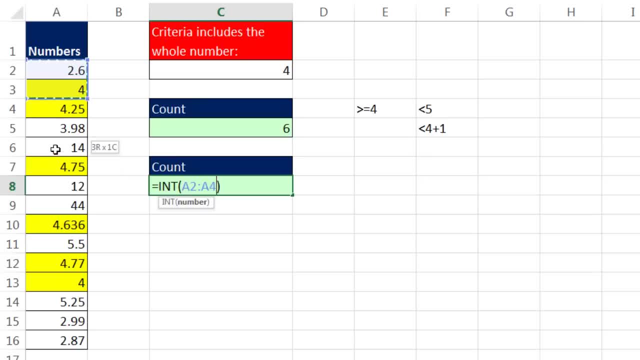 But check that out. We don't want just a single number. I'm going to highlight the entire column. Now. once you do this, that number argument there is expecting a single cell. I'm giving it a range of numbers And actually I already created a defined name here. 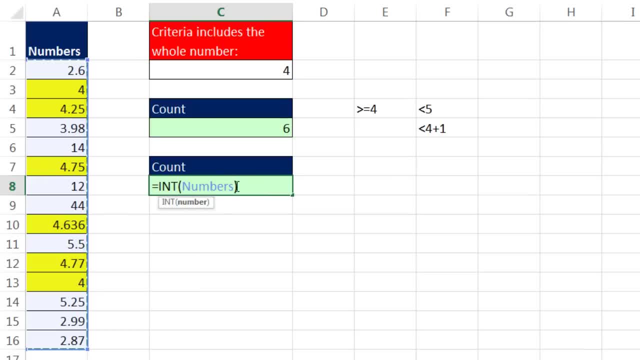 so that range of cells is called numbers. But now, if I highlight this, that's going to get me to the number. This is now going to do a what's called a function argument- array operation- because we threw a bunch of values into the number argument. 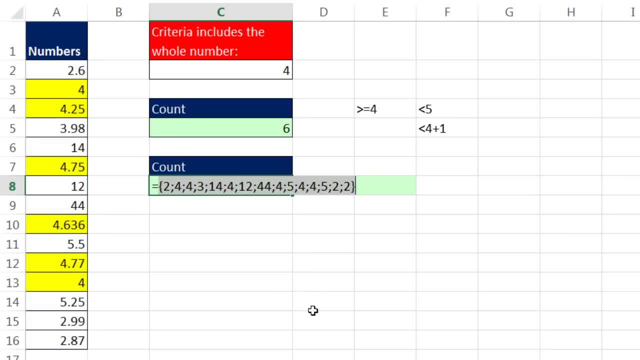 Int is instructed to spit out a bunch of answers. So when I hit F9, there it is, Now Control-Z. I want to ask the question: are any of you in that whole range that int is spitting out? are any of you equal to 4?? Now, if I highlight this and hit the F9 key, I get, oh, a bunch of true numbers. So I'm going to hit the F9 key. I'm going to hit the F9 key, I get, oh, a bunch of true numbers. 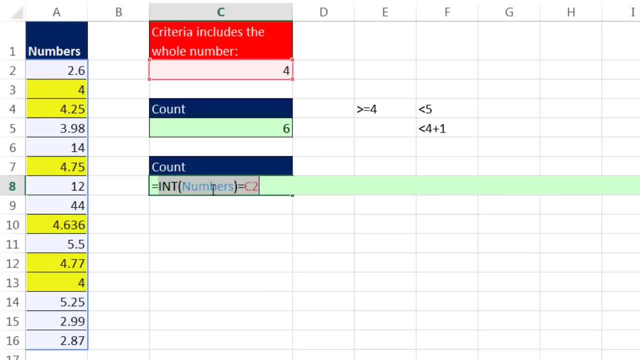 Oh, a bunch of trues and falses. Now, this is an array operation. There's two array operations. There's a function argument array operation that's spitting out an array of answers. That's why it's called an array operation. 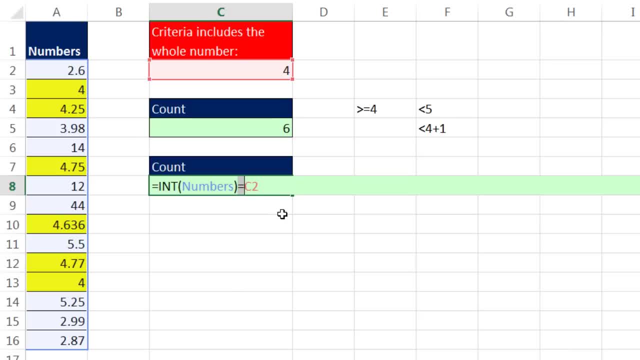 Here is an operator equal sign. It's also spitting out an array of answers. We ultimately need to add all of the trues to get 1 and the falses to get 0. So I need to convert those trues and falses to ones and zeros. 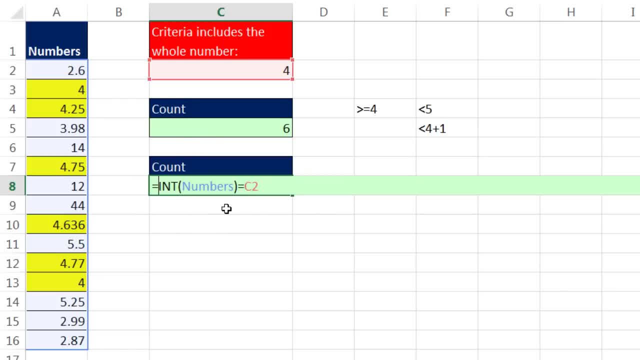 I could do this a few ways. Any math operation can convert trues and falses to ones and zeros. I'm going to choose to do double negative. It tends to be the fastest calculating Now, right now. comparative operator evaluates after a math operation. 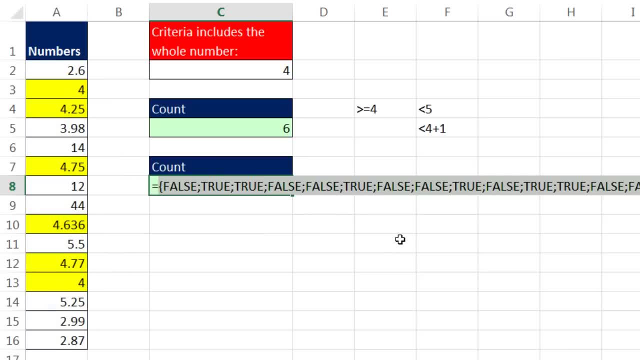 So if I were to highlight this and hit the F9, it wouldn't work at all. So I need to force the equal sign to calculate first. So I have to put the equal sign first. I have to put parentheses around here And now, when I highlight this and F9 to evaluate. 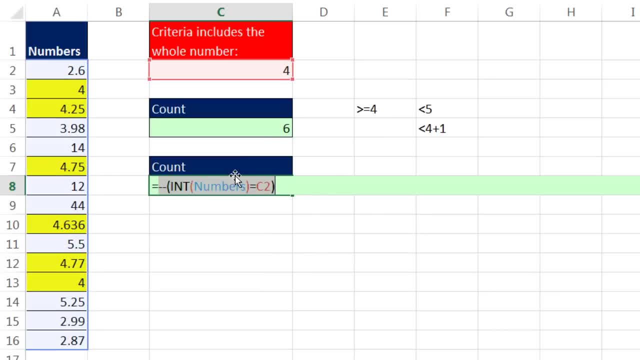 I have exactly what I need: Control-Z. Now, that's an array operation. If I put it inside the SUM function, I'd have to use the special keystroke Control-Shift-Enter. But I don't want to do that because there's 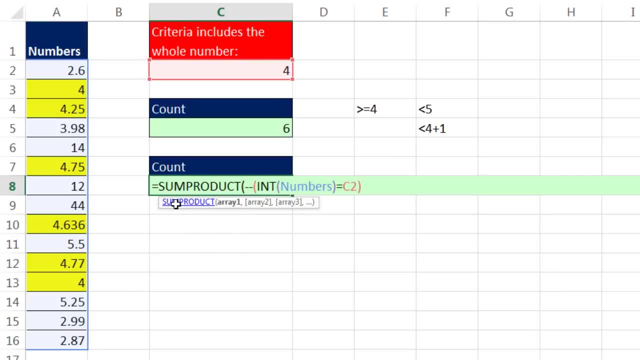 a function called SUMPRODUCT. Now, SUMPRODUCT normally takes many arrays and multiplies them- That's the product part- And then adds them- That's the SUMPART. But we're taking advantage of the fact that the array arguments in SUMPRODUCT 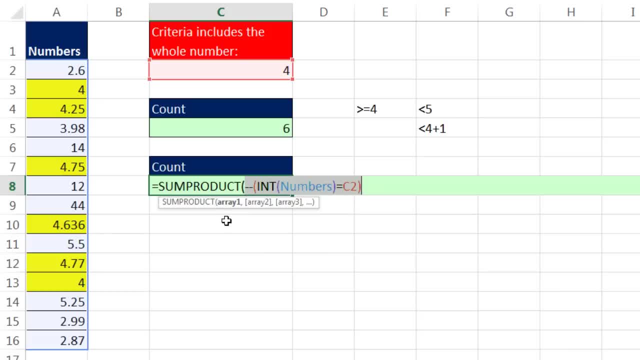 can handle array operations without any special keystroke. So it will not do the product part, because there's not multiple arrays. It'll just do the SUMPART. And there you go. Control-Enter. There are six. If I change this to three, there is one.